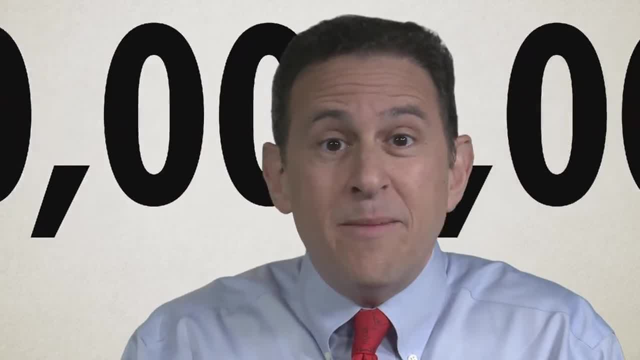 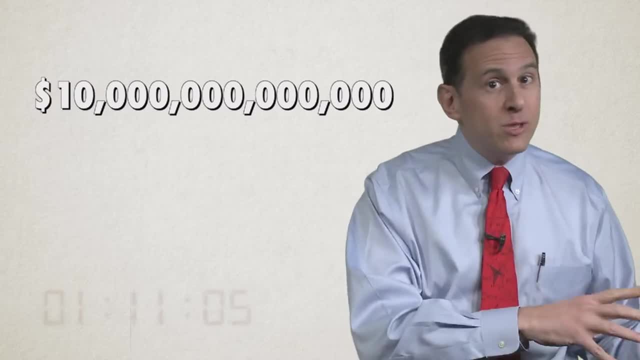 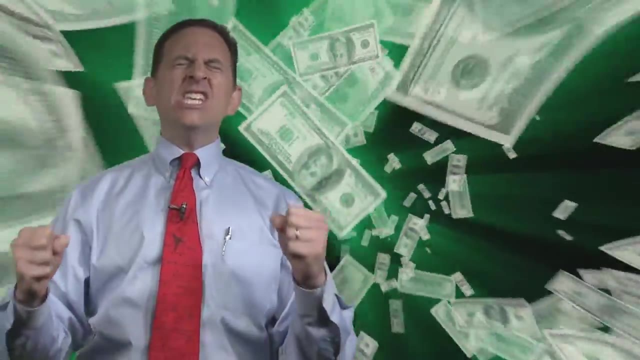 to do with that number? Nothing. you can't make sense of that number. $10 trillion is way too big for us to imagine And you can't do anything with it. But what if I now tell you that last year was $10 trillion, this year $10.5 trillion? We've had $500 billion of growth. That is enormous. in 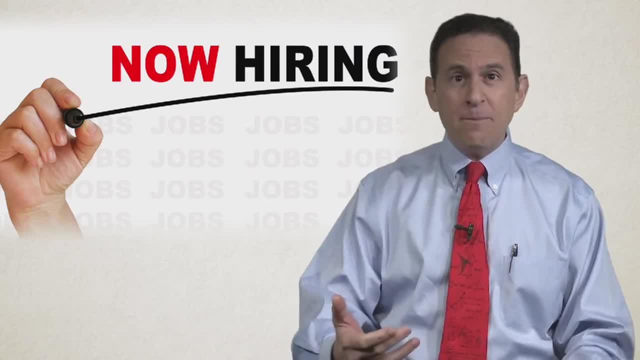 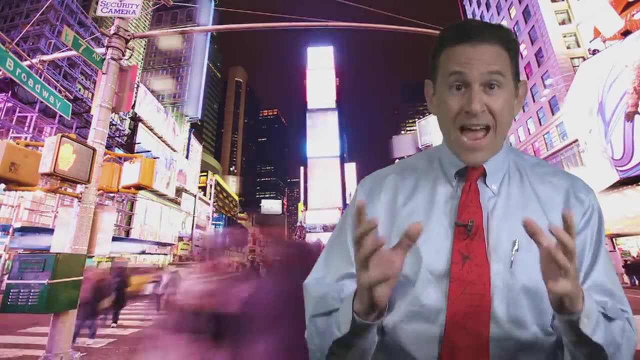 an economy like ours. 5% growth in this economy, That's everybody employed, Your housing value's gone up, Your business is opening and they're doing super well. Everybody's happy. That's 5% growth in an economy like ours. You care a lot about 5% growth. You know what you care about, even 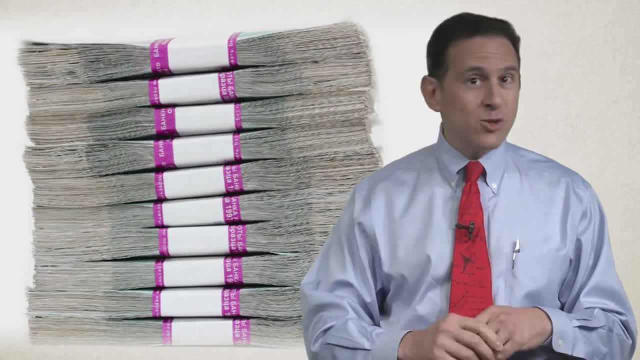 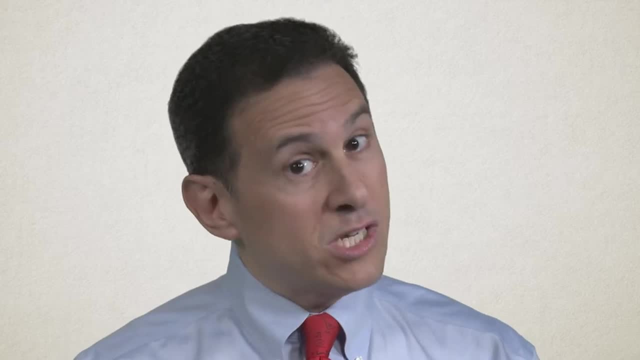 more. What if I told you, last year was $10 trillion and this year's $9.5 trillion, 5% loss. We went through something like that, not even that bad kind of recently, and we're still recovering from it. 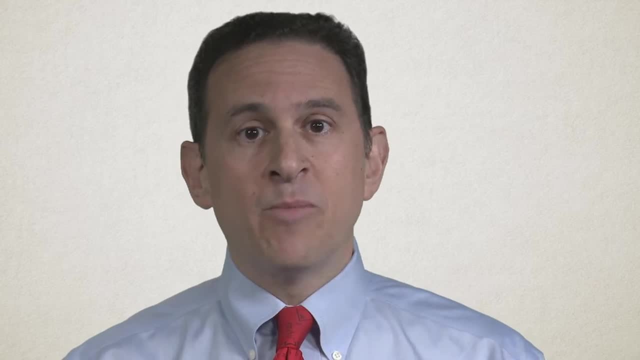 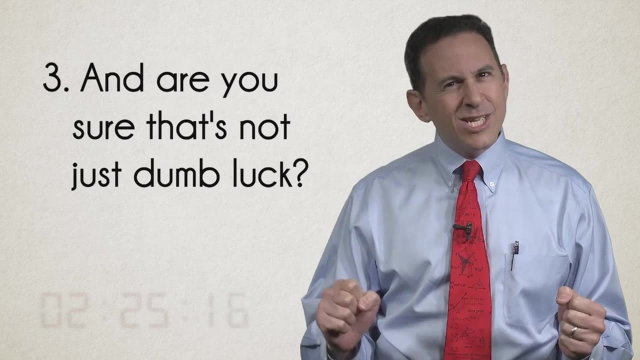 It was bad, It was not good, You don't want. You care a lot about what difference does it make? You care a lot about a 5% difference. But this brings up the third question: And are you sure that's not just dumb luck? Really 5%, You sure? 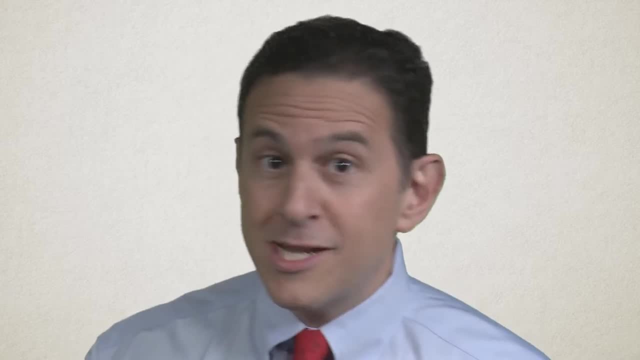 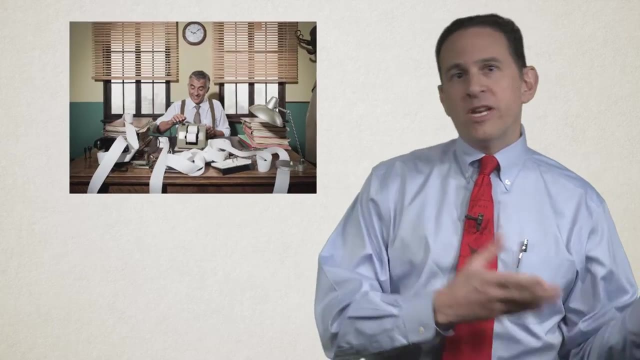 about that number? What if I told you that the $10 trillion estimate I gave you and the other estimates I gave you come not from the federal statistical system, but instead from my Uncle Bernie's research firm? Uncle Bernie, he's got a good guy, He's got a good research firm, but he's 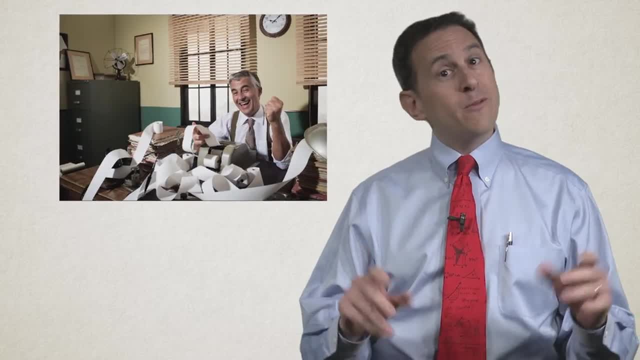 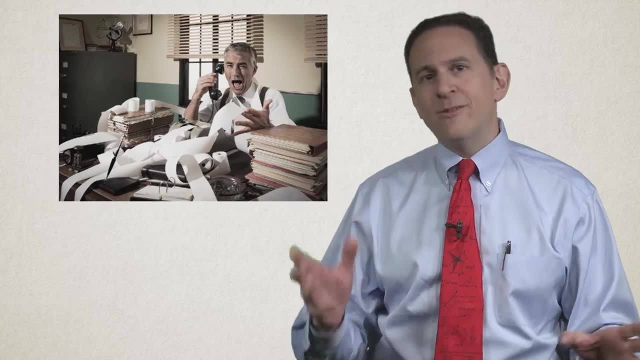 not quite as big as the federal statistical system And his numbers do not have the same precision that the federal statistical system can offer. His numbers are accurate within about- I'm going to say- $500 billion. He's giving a $10 trillion estimate, a $10.5 trillion, a $9.5. 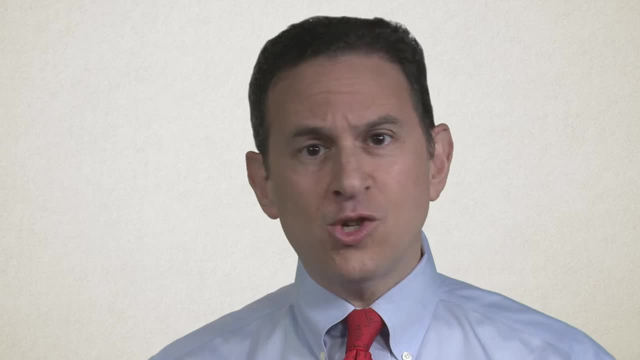 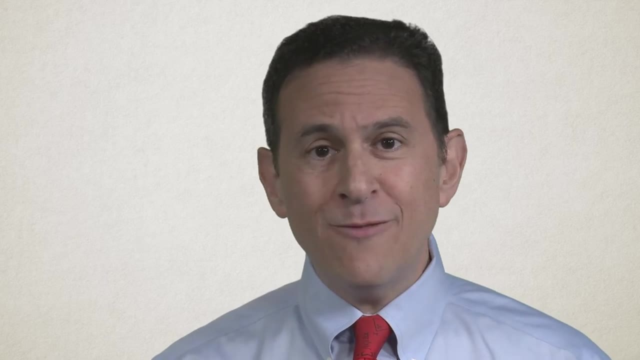 trillion. It's all with a trillion dollars of range around it. I mean the $10 trillion is just in the middle of a trillion dollar range. These ranges completely overlap. I mean there's no way to tell the difference between these numbers. Could be up, could be down, Whether it looks up. 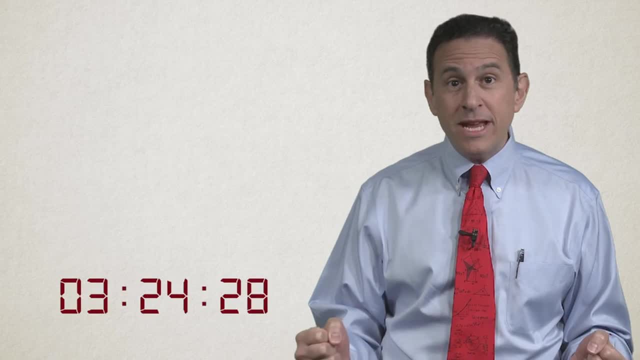 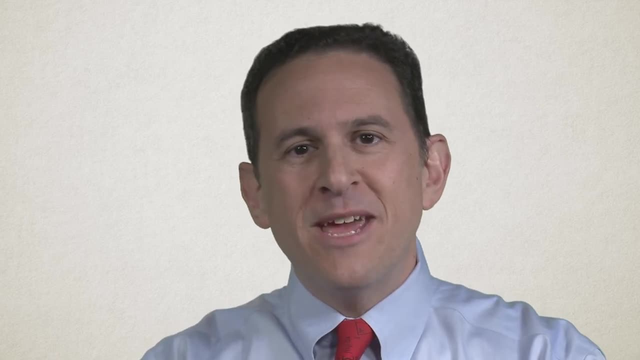 or down. So that's all of statistical analysis in three minutes. How'd I do 325.. All right, Okay. So how big is it? What difference does it make? And are you sure that's not just dumb luck? Often answered with math, but not always. You can answer them in other ways.